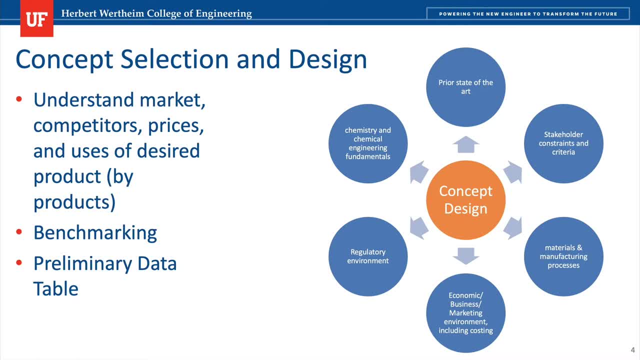 And the manufacturing process that you can use potentially in your design. Then as you progress in your design, you start doing some preliminary economics, some business and marketing studies and understanding the environment, including some initial costs. okay, And costs can be cost of raw materials right in the early stages. 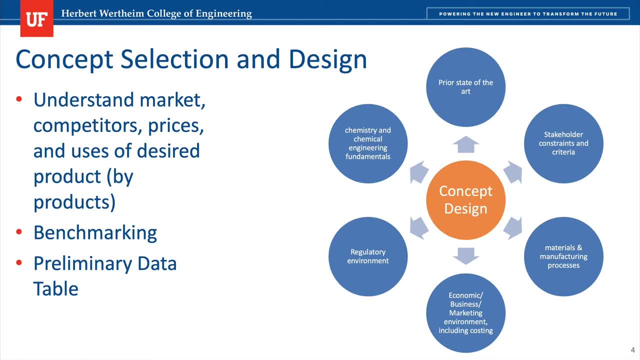 And as you progress, it could be the cost of utilities, the cost of equipment and so forth. Then all of that should be complying regulatory environment. This could be regulatory environment in terms, In terms of safety or environment on human health, or aquatic or environmental. 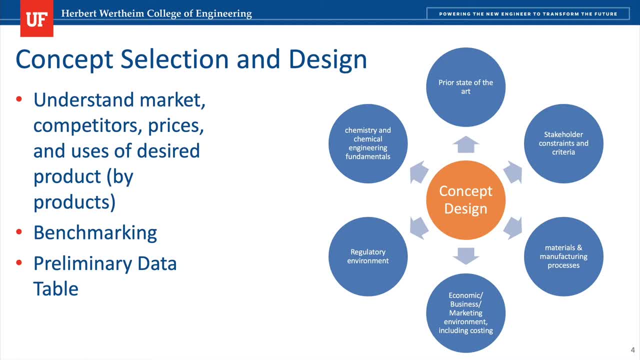 This is important because, as you refine and you create your concept, you're going to be optimizing all of this using these different constraints and different areas right on the concept, design And then finally, or initially, right. everything is embedded between all of this: business aspects and designing aspects, but always taking the chemistry and chemical engineering fundamentals as a stepping stone for your decision. 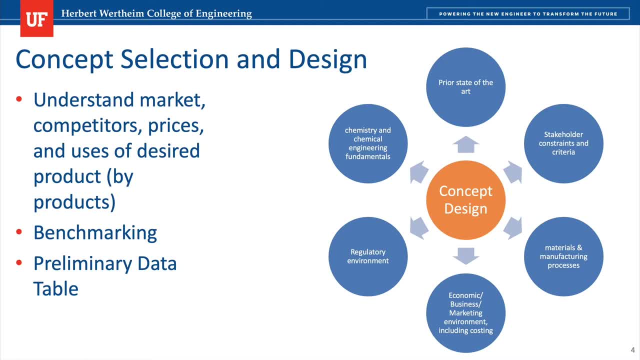 This means that you cannot violate right any law of thermodynamics. You cannot come up with things that cannot be created right, So you really need to understand your chemi fundamentals. So, as I mentioned before, we're working on example with the vinyl chloride monomer. 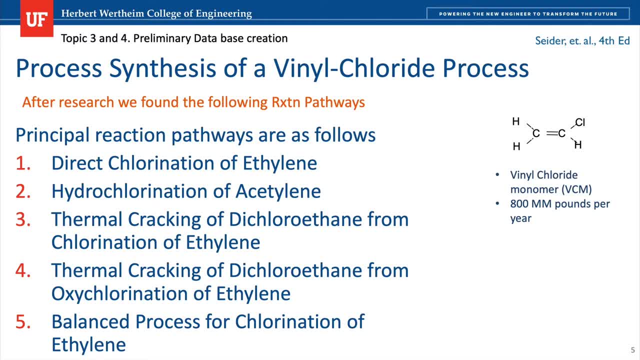 Here: when you do research- initially- right, you're doing benchmarking- you come up with multiple reaction pathways. In my class I recommend to have around 10 reaction pathways And the idea is that you see what is out there. Sometimes you neglect some of these. 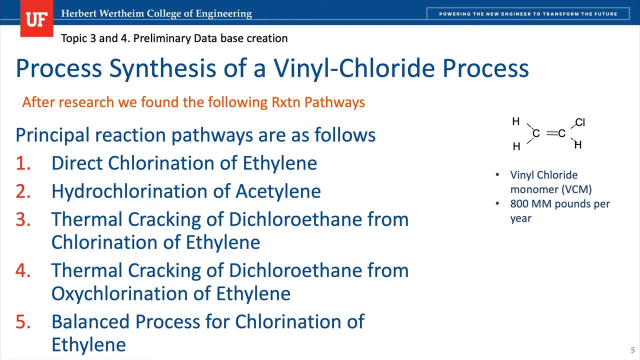 Sometimes you neglect some of these reaction pathways, but sometimes, by reading the separations or maybe seeing how they handle side reactions or byproducts, you may come up with new ideas in the meantime. So this is the example: right with this vinyl chloride and I have five reactions. 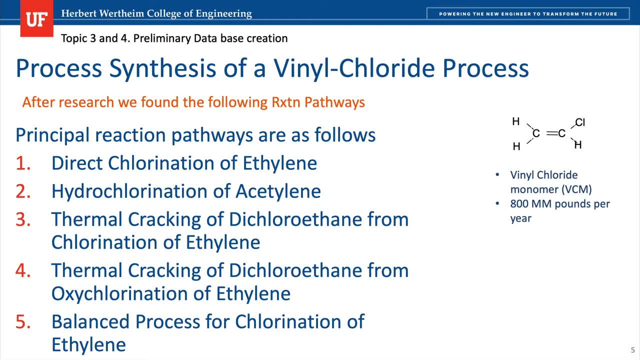 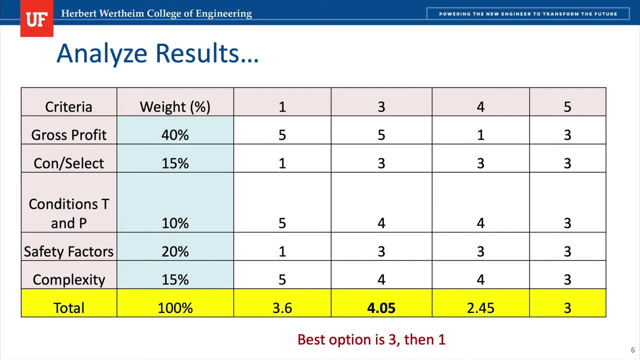 And from those five reactions I went through a process of selecting which one is the best right. We went through a screening table and a scoring table. From there, we analyzed the results and we found out that reaction pathway three And reaction pathway one may be the top candidates. 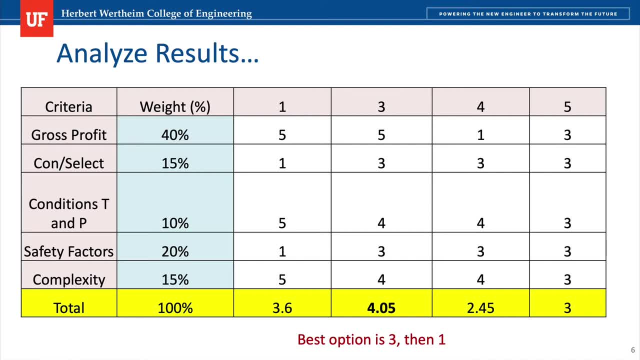 And we like to have two candidates, just because when you go to the simulator sometimes you realize that you cannot simulate one over the other. But either way of the two you pick, you know that it is the best option, based on the different criterias, that you select it in your concept as selection process. 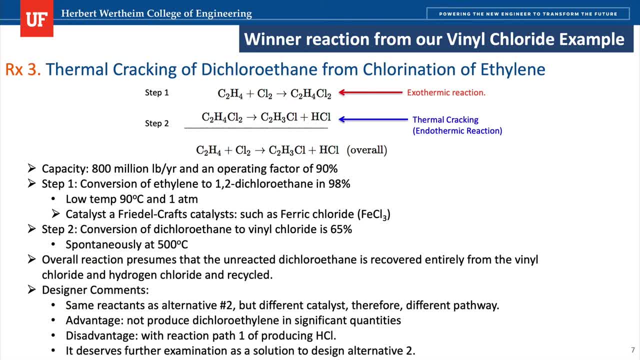 So when you find out the winner reaction from your scope of work or for your particular process, you need to go back again to the last one literature and make sure that you have enough information to be able to simulate it So you can have the best chemical reaction and the most profitable chemical reaction. but if we cannot, 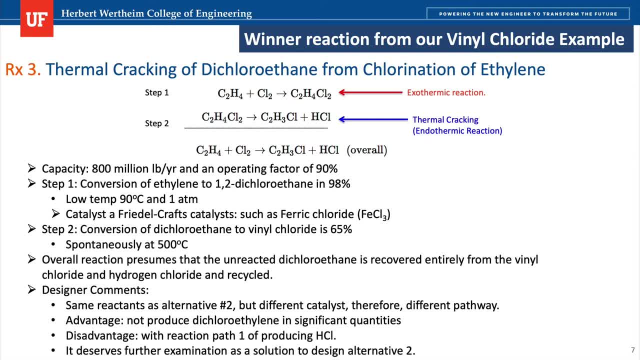 simulate it with the tools that we have. it may be a problem, right, to understand the scale-up, particularly in a project that has time frame, like the ones that we do in this in my class. right, We do a process design. we have around 15 weeks to complete the project, so we have to make. 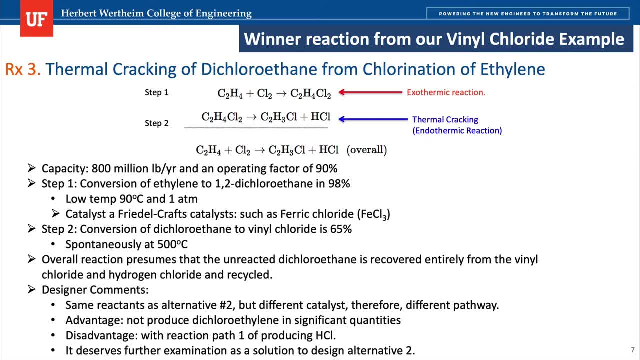 sure that we can simulate it using the tools that we have available. Remember, always have information about the capacity, information about the specific reactions. If you have two reactions, two different steps in the reaction, that means that you're going to have two distinct reactors. 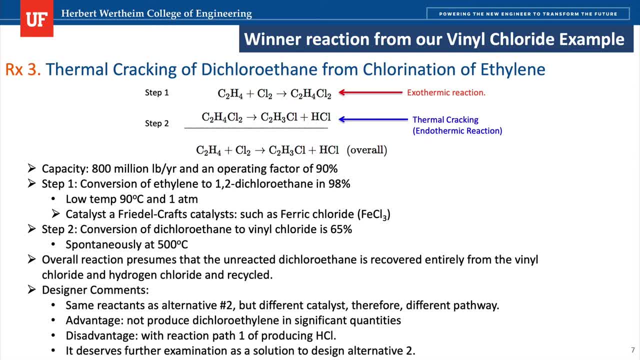 In one reactor you can have side reactions, so that will happen in the same reactor. So you need to understand right the conversion, the selectivity and all that for your particular reaction. Then you need to have information That you can get in the literature. maybe you have information about which component is in. 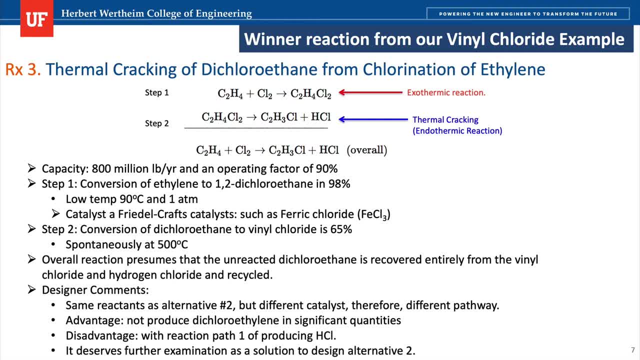 excess. you may have information about the residence time or the volume of the reactor. Either of that information is important, especially when you do sizing later. Then you kind of summarize the designer comments just to remind yourself of the important aspects of this. 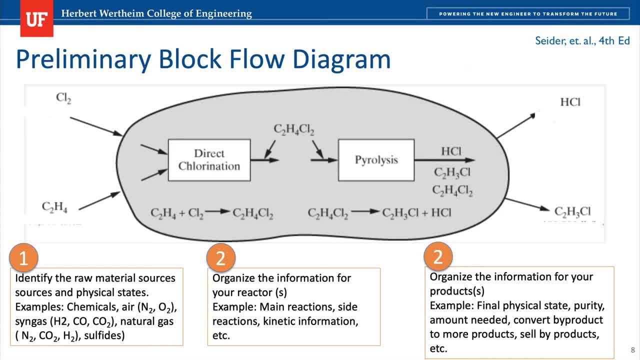 chemical reaction. So when you start building, before you start simulating, the first thing that you do is to create a preliminary block flow diagram. This is a very holistic overview of what the design will look like. I like to do this in a piece of paper or maybe on a presentation. 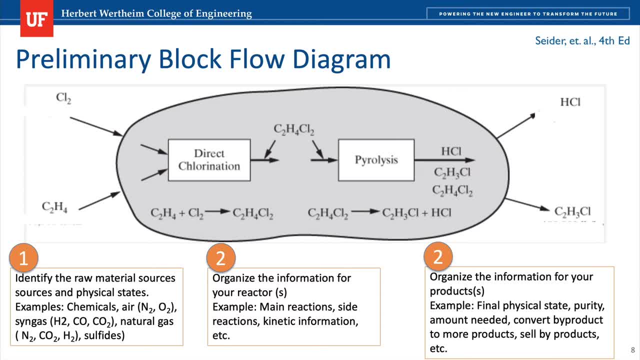 slide And the idea is that you can envision where is your goal right. So you need to identify the raw material sources and physical states, The react, the raw materials. they must come into the system as we find them in nature If you need to process them and pre-treat them before adding them. 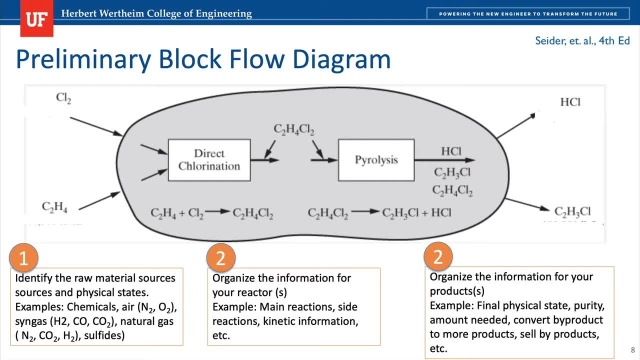 to the first reactor. that's perfectly fine, But it should mimic right what is out there and how we're going to get the source of that raw material. So that is an important design parameter. You can also have besides rock like the actual. 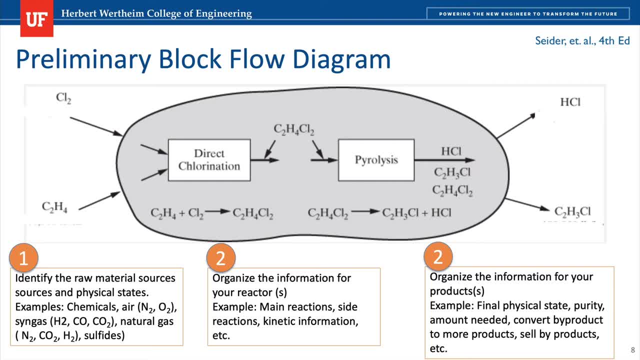 chemicals, let's say chlorine or ethylene or whatever chemical you have here. You also need to consider other sources, right, You may have, instead of purchasing pure nitrogen or oxygen. maybe you want to use air. right, It's readily available, So you just need to add a separation. 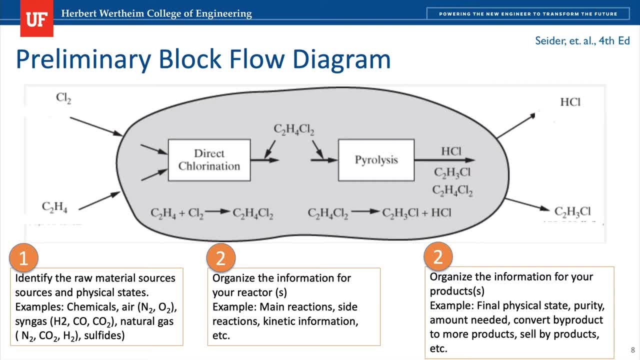 unit, Probably cryogenic to separate the nitrogen from the oxygen. But I mean air is cheaper than purchasing the nitrogen and the oxygen. You also have to consider you can also consider syngas. right, That is synthetic gas or natural gas. All of them have different compositions of. 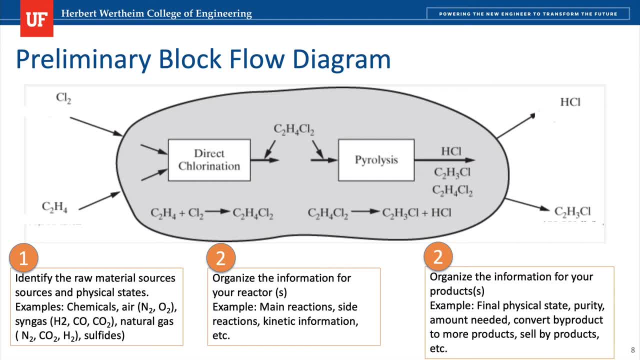 maybe reactants or building blocks- right That you can use Smaller molecules right are considered to be like building blocks And you can find them in different ways. Then the second is back again organizing, So having clarity in terms of the information for your reactor. main reactions, like reactions. 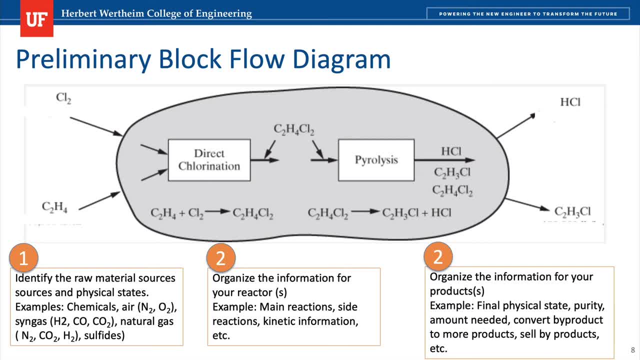 kinetic information, information, et cetera, et cetera, Anything, information in terms of the excess, if there are added in stake-a-metric amounts, so forth. And then you organize the information for your products. You need to know the final physical state, right, You're not gonna sell. 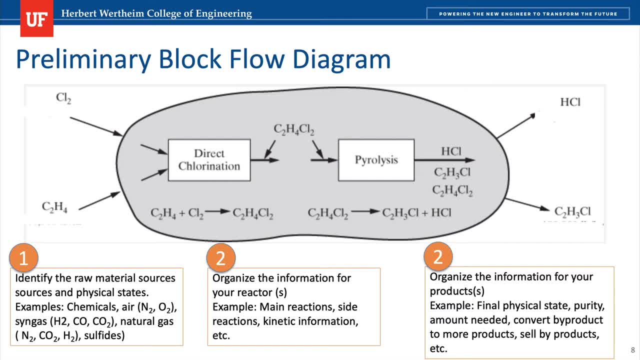 hot HCL gas right. You need to make sure that the way that you're gonna be selling this is gonna be the way that is coming out from your process for diagram. once again, find out physical states, the purity, the amount needed, particularly of the desired product. convert any byproduct to more. 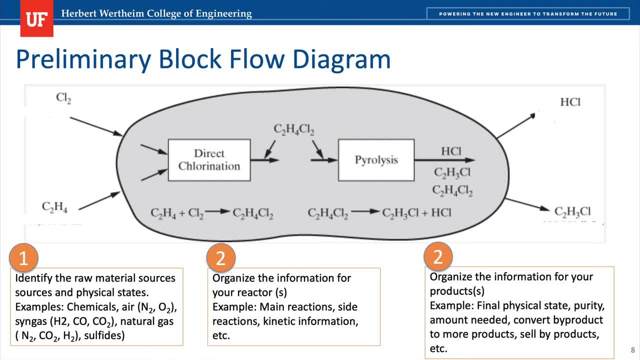 products if you can right. the target is to produce the desired products. if you have a byproduct, try to find ways, instead of this post set, to actually convert it into more product, because that's the target of your project. and if you can sell all products or buy products, if you cannot, uh, mitigate. 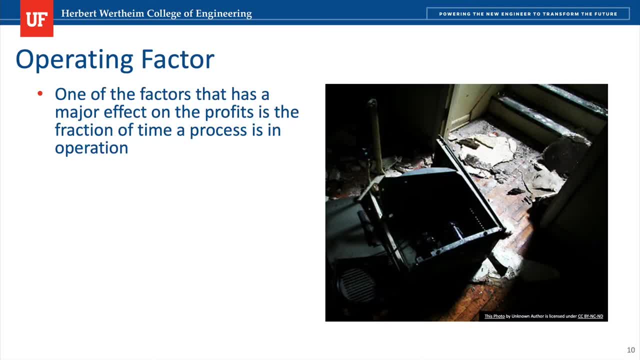 it mitigate them or treat them. the operating factor is one of the factors that has a major effect on the profits and it's basically the fraction of time a process is in operation. anytime that a plan is not producing a product, it is also not producing revenue. downtime in. 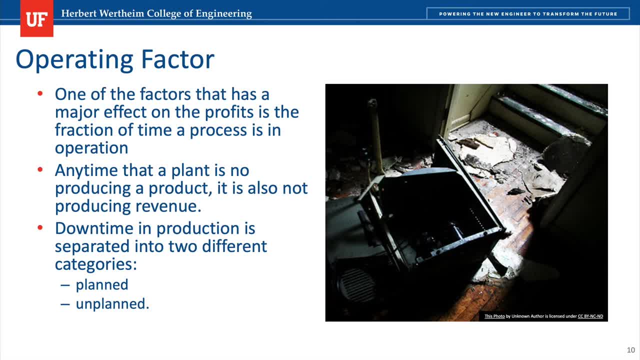 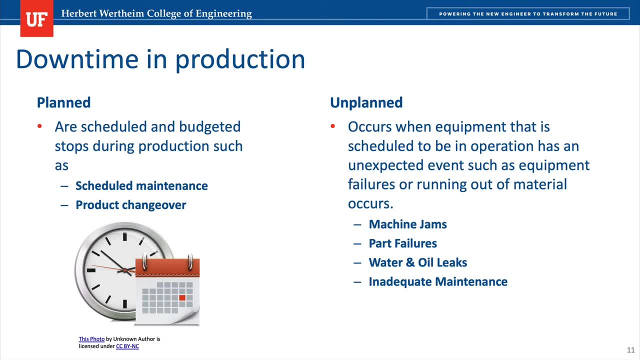 production is separated into two different categories: planned and unplanned. when you're dealing with planned downtime, these are typically scheduled and budgeted stops during the production, such as schedule maintenance and product change over. so let's say that you need to maintain your production and you need to maintain your production and you need to maintain your. 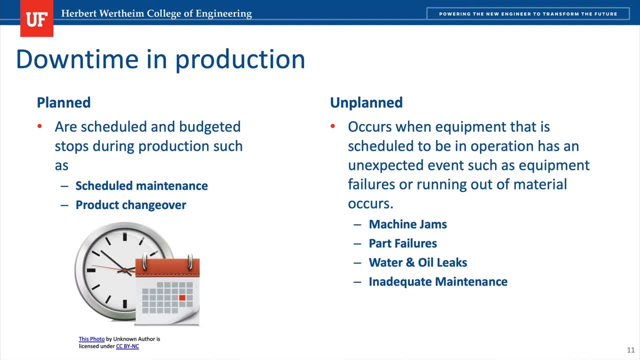 turbines because you're producing energy out of steam. so you can schedule that maybe twice a year, right every six months. you can also change products in line. let's say that you're in a pharmaceutical company and you're producing two different drugs and every six months you rotate between one and 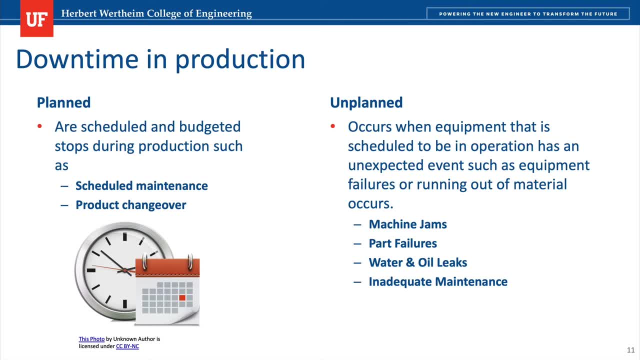 the other right, or you have a schedule every two weeks or depending on the type of product. but product changeover is really common in all industries so it has to be added into the calendar and planned also. there are a number of different ways to change the product so you can change the. 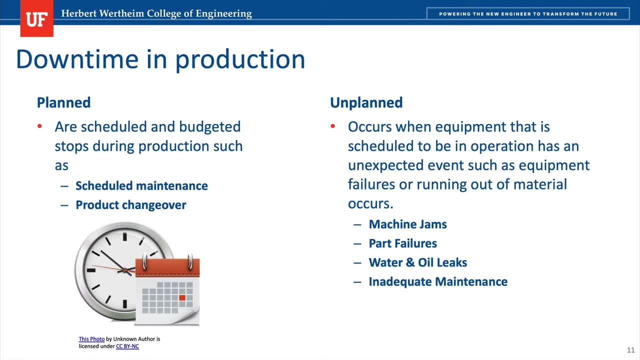 there could be unplanned downtime productions, and these are undesired. they occur when equipment that is scheduled to be in operation has an unexpected event, such as an equipment failure or running out of materials. you can have also machine jams, part failures, water and oil leaks. inadequate maintenance: let's say that you schedule something to maintain but then something. 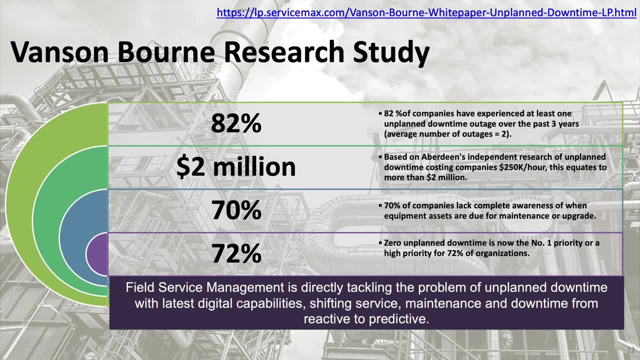 happened that didn't go well. following the vanson burn research study- uh, the reference is here. uh, you can find that around 88 percent of companies have experienced at least one unplanned downtime outage every over the past three years. the average numbers of outage are two, based on an independent. 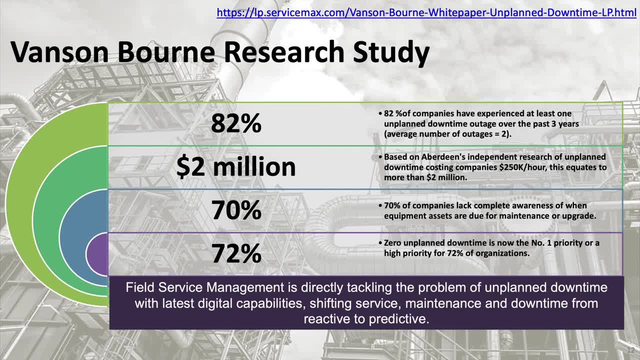 research, they found that downtime end up costing companies around 250k per hour. this equates to more than two million. so this on-plan downtime is important, right? this translates into economical losses. seventy percent of companies lack complete awareness of when equipment asks for maintenance or upgrades. so having a system in place can actually save some money at the end. 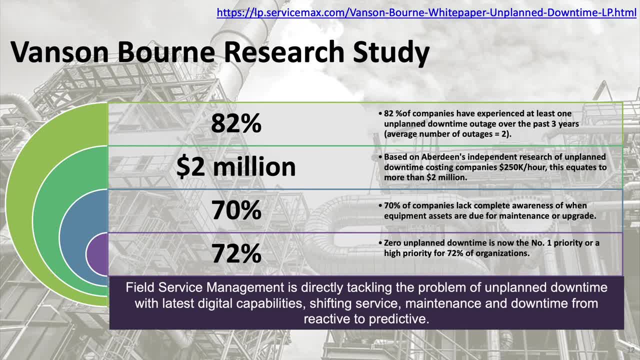 zero on-plan downtime is now the number one priority, or high highest priority right of around 72 percent of the organizations interviewed in this study. remember, fuel service management is directly tackling the problem of on-plan downtime with uh, basically with late latest digital capabilities, shifting service maintenance and maintenance to a more sustainable way. 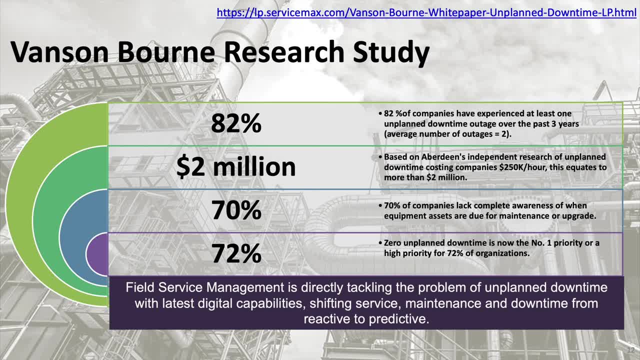 of operating the system. so this is an example of a lot of the things that we've seen in this study. so the first one is the cost of maintenance and downtime. from reactive to predict, predictive, so a lot of things here in terms of process control, uh, artificial intelligence trying to. 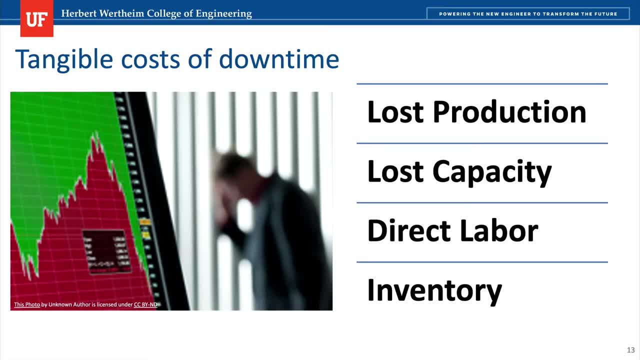 understand the data of production to be able to predict right when this downtime happens and be proactive instead of reactive. there are multiple costs associated to downtime. the first one is of of capacity right, the total amount of capacity that the plant can target if your process is designed to produce a certain amount of product and now you are producing less because you have 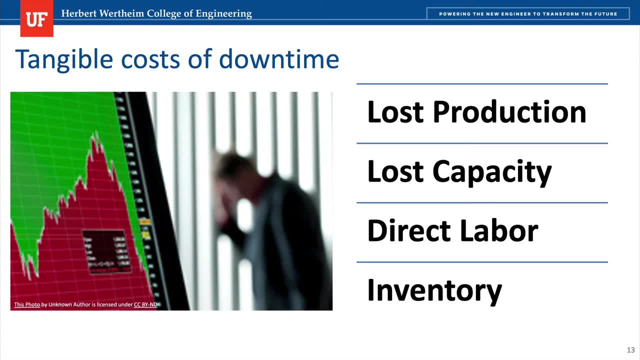 some equipment down. that means that it will impact the sales too. also, it will impact- uh it can impact- the direct labor. direct labor can be more costly because if you have a personnel in the plan but you're not selling anything, that means that the cost per labor. 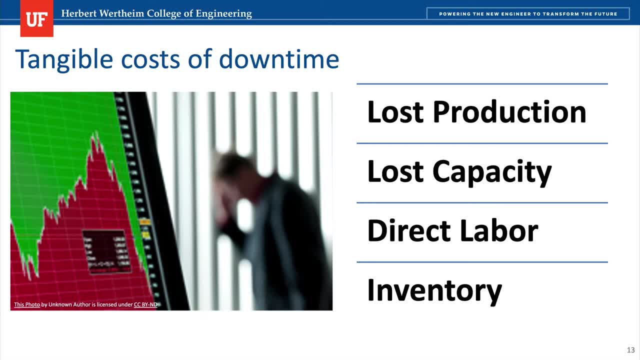 will be increased as compared to the amount of sales or profit of the company and also the cost of storing the inventory. right, if you have the raw materials because you're not using it, because the capacity is down, you have to pay for that. anything in the inventory in the inventory means that it's 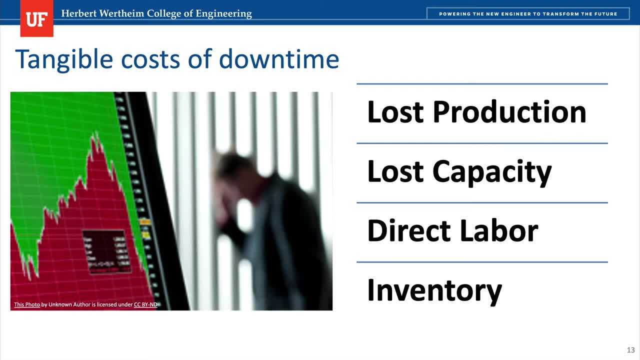 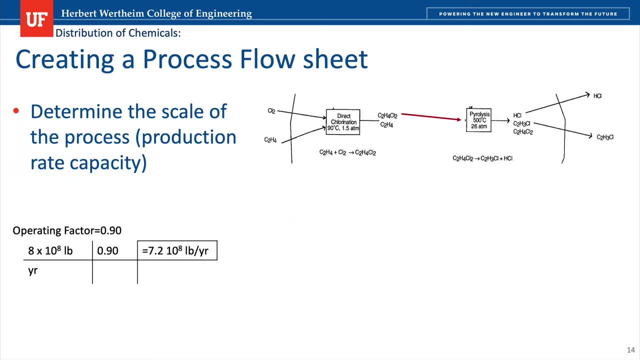 not being sold. so if it's not sold, that means that there's no money coming in and there's no profit. so it is important right the operating cost and uh taking that into consideration. so we design our plan accordingly. when we we are creating a process flow sheet, first we determine the scale of the process. 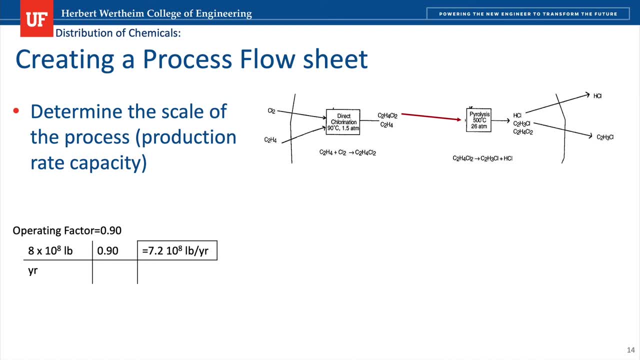 and the production rate, capa, or the production rate capacity. we know, for example, for this particular statement, that we the operating factor is around 0.90. right, it's the 0.90 of the total days of the year is when the plan is in operation. you can multiply the capacity of the plan, the 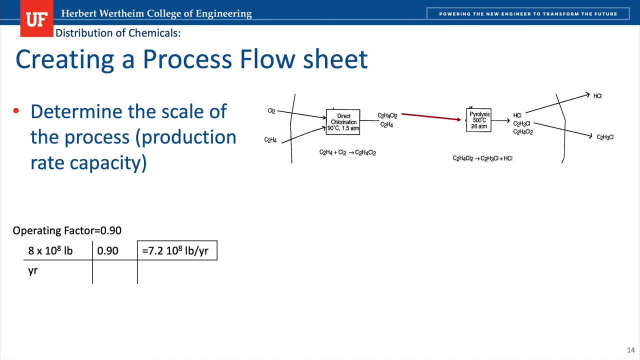 target capacity of the plan for the product and that will tell you how much the downsizing right on capacity will be due to the process and the capacity will be due to the plan's scheduled downtime. this translates right into 101 and 500 pounds per hour and we transfer that into pounds per hour because usually these are the most common. 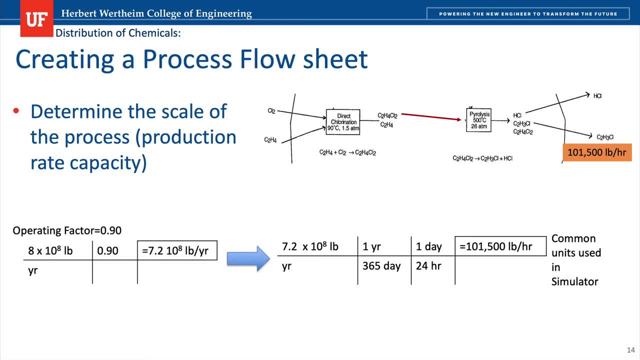 units using simulators. however, simulators can convert units from one and the other. i'm more used to use pounds per hours or kilograms per hour if you're changing units to the si system. the thing is that all of this number translates into cost losses. right, we don't want, we need to. 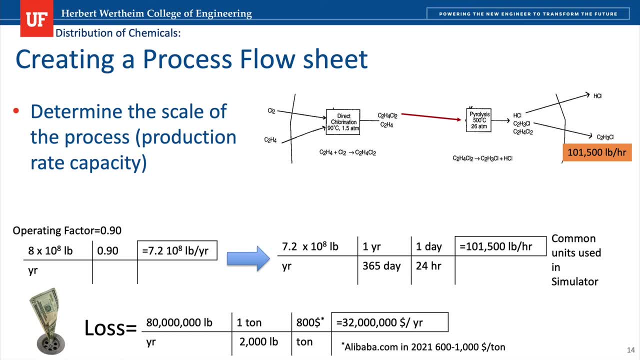 know that because we need to plan, instead of producing the target amount, that we're producing less, because we have to plan for that. that means that we're losing around 32 million dollars per year, right, or things that we could have sold right, if we have the 365 days of work of the year. so it 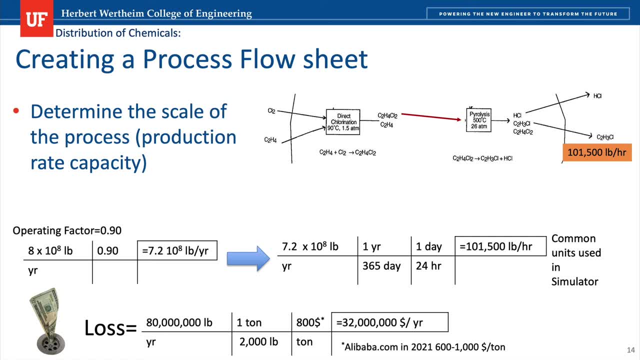 is important to consider right the process flow sheet in the plus a flow sheet, the operating factor. this will impact the scale of the process, the size of the equipment, the amount of utilities of raw materials. everything in the economics right will be affected by the scale. so this: 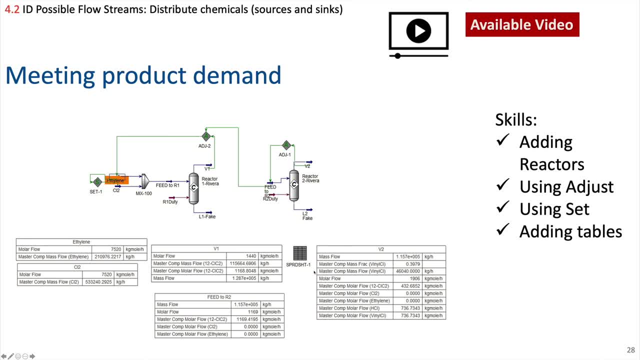 initial part of this video right. basically, at the end of the day, what you want to make sure is that when you add your reaction scheme, you have all the information to input that into the reactor. it could be a conversion reactor, a kinetic reactor, equilibrium reactor. then you can not only talk. 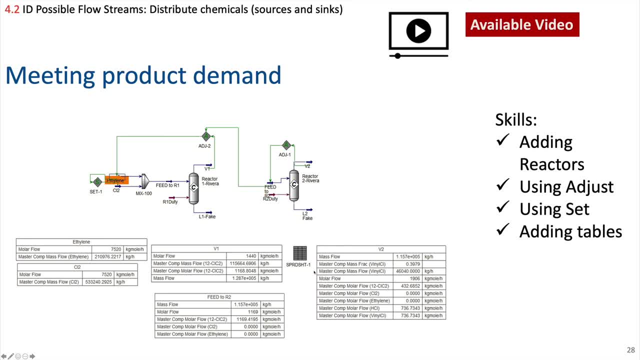 about the type of reaction, but also type. talk about the type of reactor. it could be low flow reactor, a cstr. uh, it could be a packed bed reactor. there are different type of reactors that you can pick And there's also a couple of functionalities.